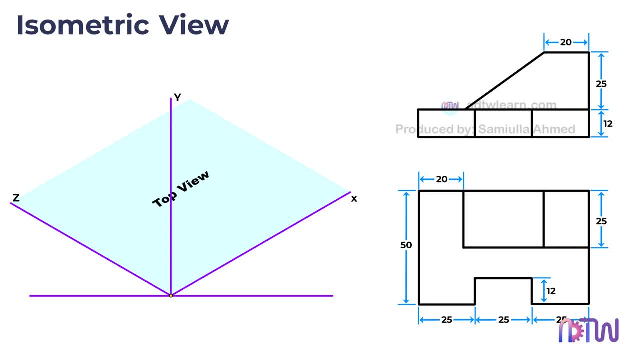 the x-z plane. so that's another key point to keep in mind. Since we will be using the first angle method to solve all the problems, the top figure will be the front view of the object, while the bottom figure will be the top view of the object. 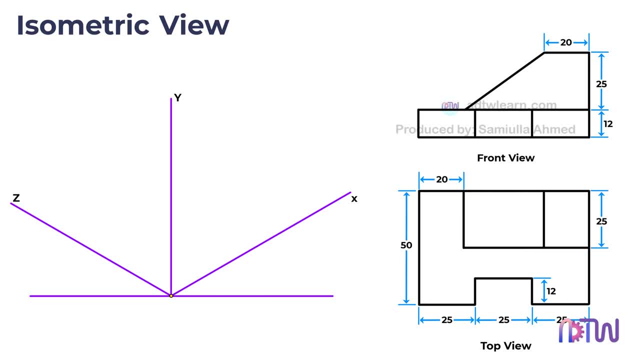 The x-y plane's important points will help us accurately construct the isometric view of the object. We will draw the front view of the object in the x-y plane, as this will make more edges visible. We will start by drawing the top view of the object, which always comes on the x-z plane. 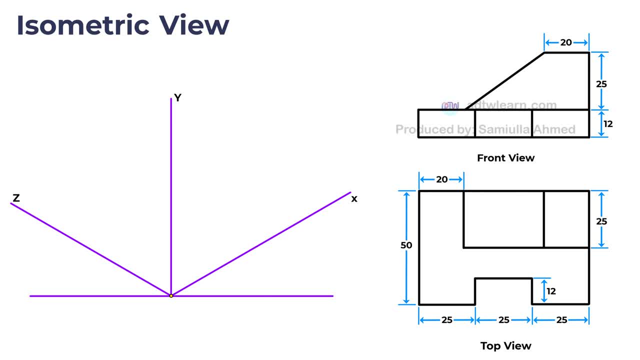 To do this, we will first draw the outline of the object. From the given orthographic projections we can see that the total length of the object is 75 millimeters and the width is 50 millimeters. Therefore, we will draw a rectangle of 75 millimeters. 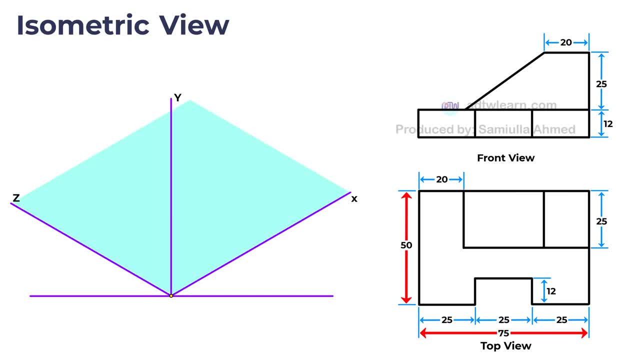 in length and 50 millimeters in width on the x-z plane to represent the top view of the object. Now that we have the outline of the top view, we can move on to constructing the features of the object. From the given orthographic projections we can see that there is a 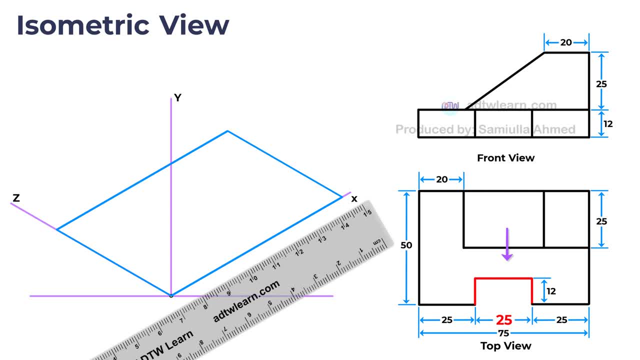 slot on the top of the object that measures 25 millimeters in length and 12 millimeters in width. To construct the slot on the top view, we need to locate its position. on the outline, We can see that the slot is 25 millimeters away from the edge. 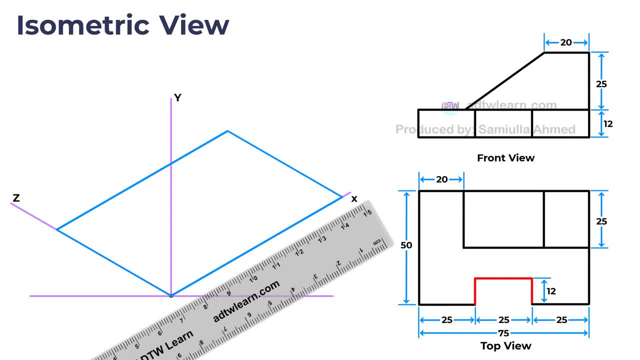 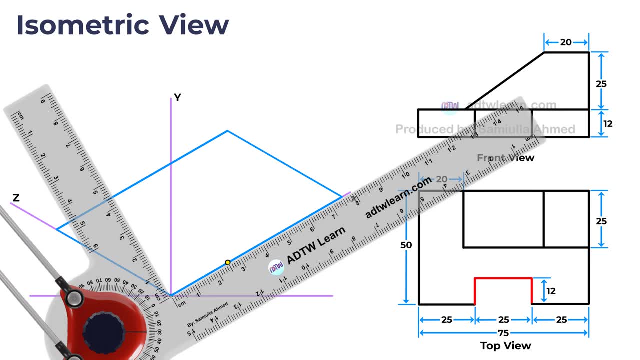 To mark this point, take a drafter and measure 25 millimeters from the edge. Mark a point at this location. Then measure another 25 millimeters from this point and mark another point. Next, align the drafter parallel to the z-axis and draw a parallel line of 12 millimeters from each of the points you marked. 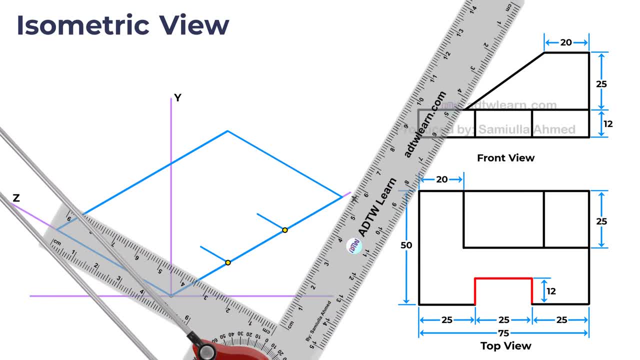 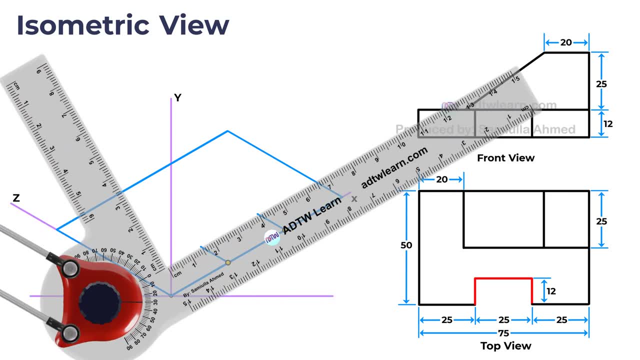 Finally, join the two points you marked to complete the slot on the top view. These lines should be perpendicular to the edge of the outline. Finally, join the two points you marked to complete the slot on the top view. This is the outline of the top view. 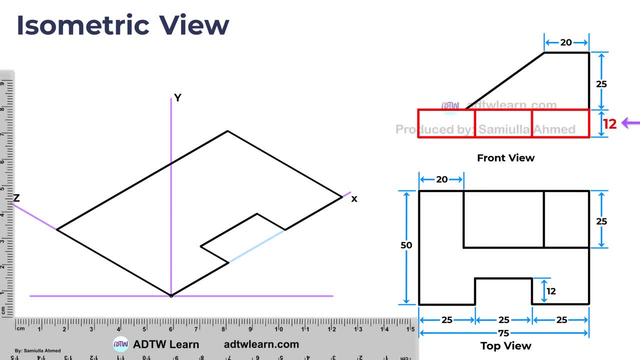 We can see from the front view that the base has a thickness of 12 millimeters. To represent this thickness in the top view, we need to increase the thickness of the outline by 12 millimeters Using a drafter, extend each edge of the outline by 12 millimeters vertically. 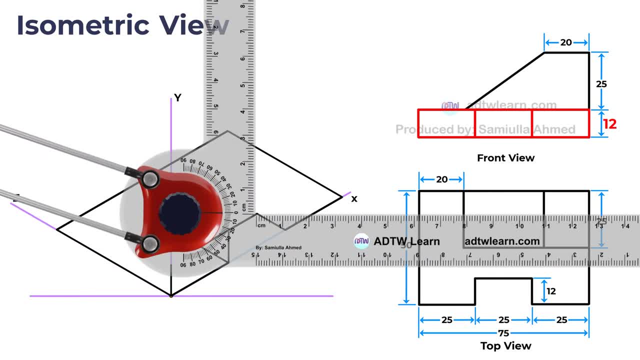 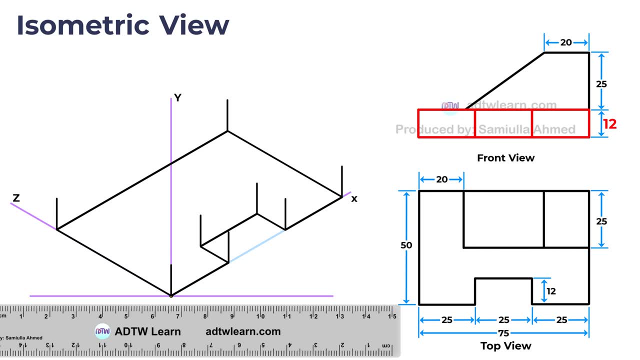 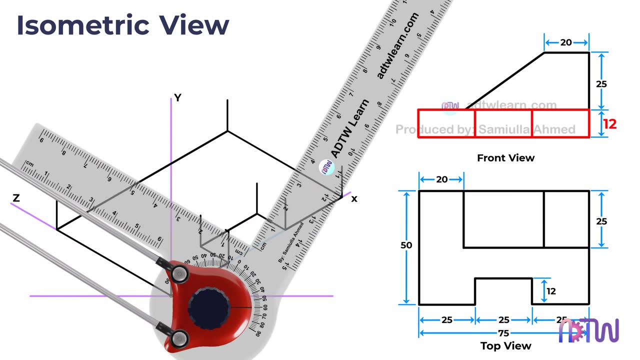 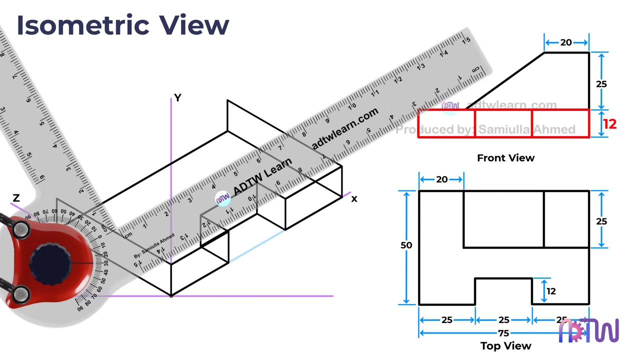 In parallel, grind it back and forth to into his bottom view. If we are to make a single drafter, next place the longer ones at each edge, and then vocês podem fazer a conосco mais longo. In this case, you might want to connect a 4mm sound line to the top view. 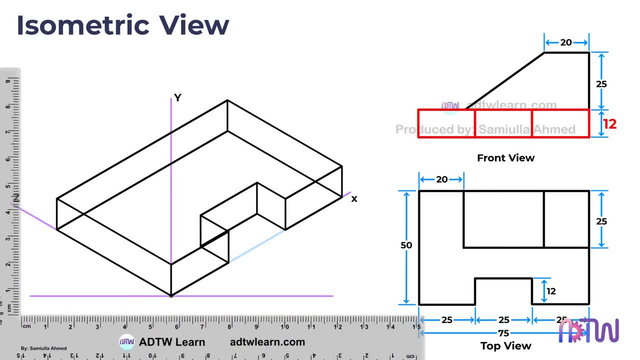 which is a 3.5 flange breaker. Next, we need to join the endpoints of the extended vertical lines to complete the outline of the base for the isometric view. Next, we need to join the endpoints of the extended vertical lines to complete the outline of the base for the isometric view. 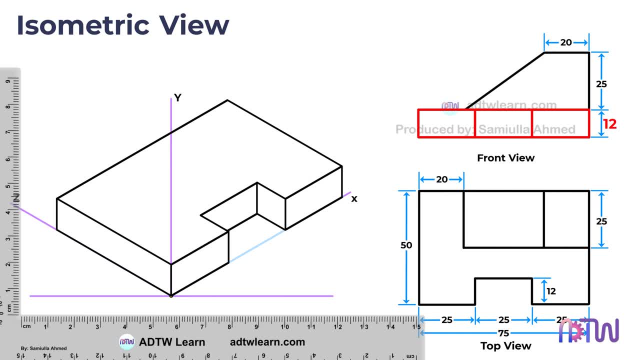 view, We can now remove all non-visible lines from the base to make it clearer and easier to understand. Moving on to the next step, we need to construct the top portion of the object. From the top view, we can see that the top portion is a rectangle that is 20 millimeters. 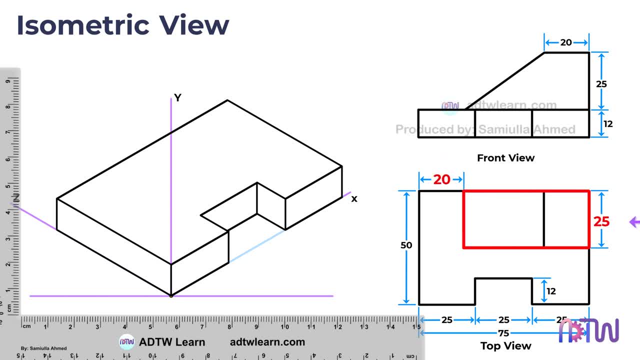 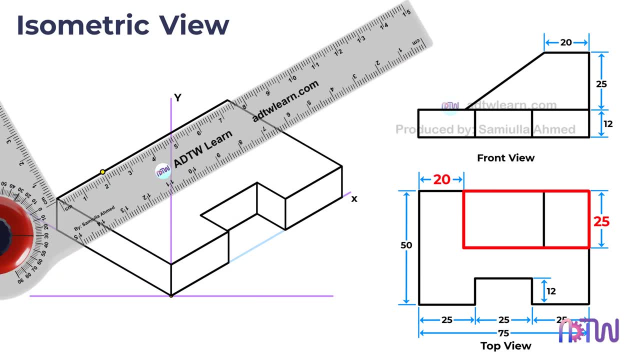 away from one of the edges of the base and has a width of 25 millimeters. Using a drafter, mark a point 20 millimeters away from the edge of the base. Next, draw a parallel line of 25 millimeters in length to the z-axis from this point. 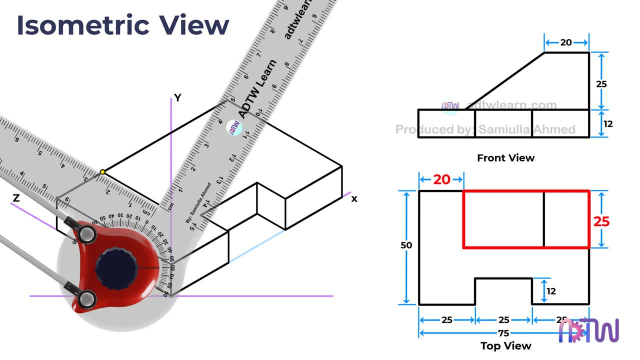 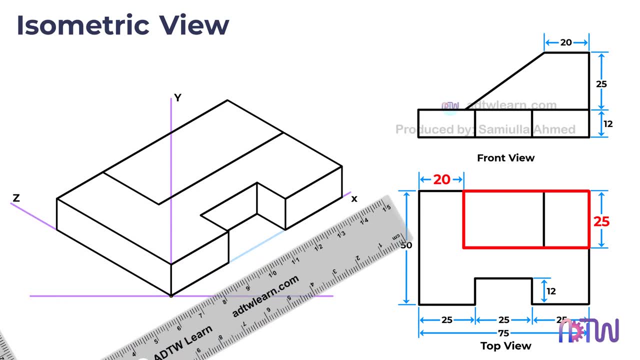 And after this draw a parallel line to the x-axis from the end point of this line as shown. This is the outline for the top portion of the object. Here we can see that this rectangle has a length of 20 millimeters and a width of 25 millimeters, with a height of 25 millimeters. 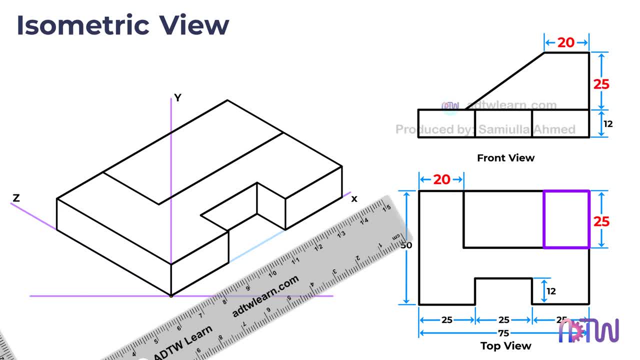 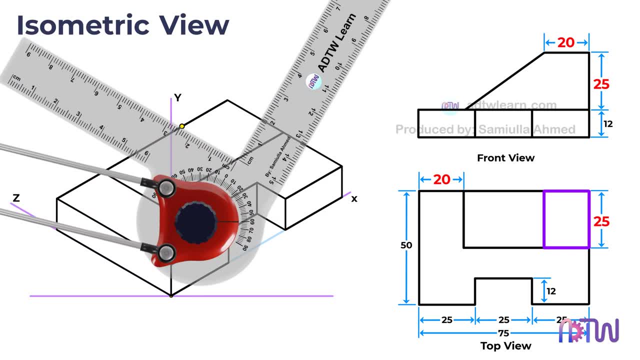 from the base. To construct this rectangle, we need to draw a parallel line of 25 millimeters. Take a drafter and mark a point at a 20 millimeters distance from this edge. Then extend the corner points of this rectangle by 25 millimeters vertically. 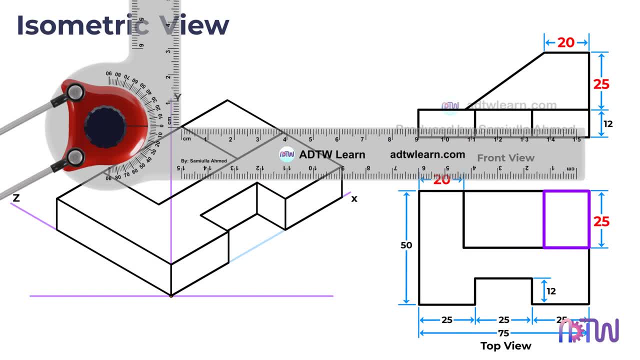 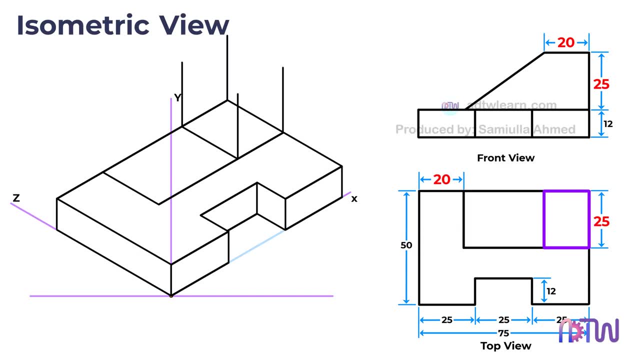 since the height of the rectangle is 25 millimeters. After this, join the endpoints to construct the rectangle. Next, we need to construct this portion of the object We can see from the front view. this portion of the object is inclined, Therefore, to construct this. join these points to these. 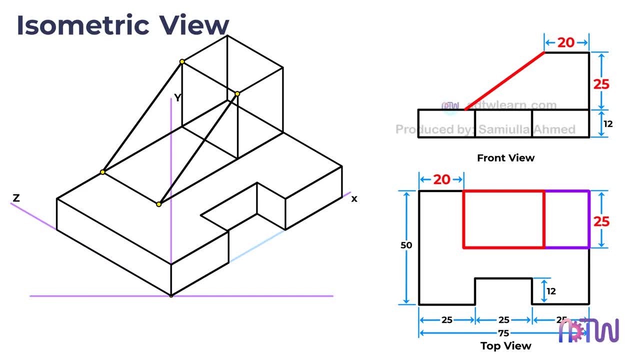 In the end, we will remove all the non-visible lines from the drawing. This is the final isometric view of the object. I hope this tutorial helped to understand how to construct a rectangle. If you have any questions, please leave a comment below. Thank you for watching.